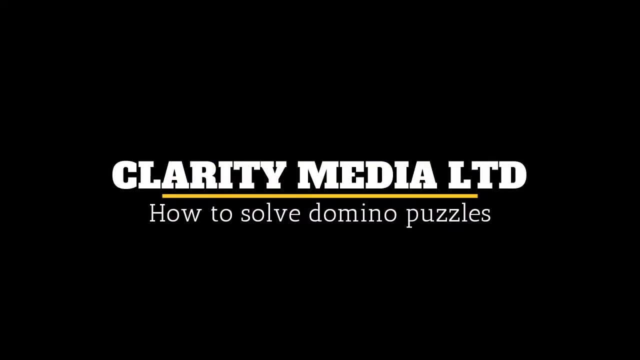 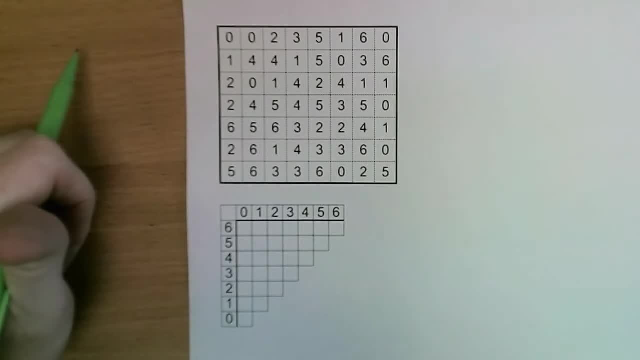 Hello and welcome to a new video in which we're going to look at how to solve a one-player domino puzzle. Now, the aim of the game is to separate this grid into 28 domino pieces representing each of the combinations from 0-0 through to 6-6, and this grid is used. 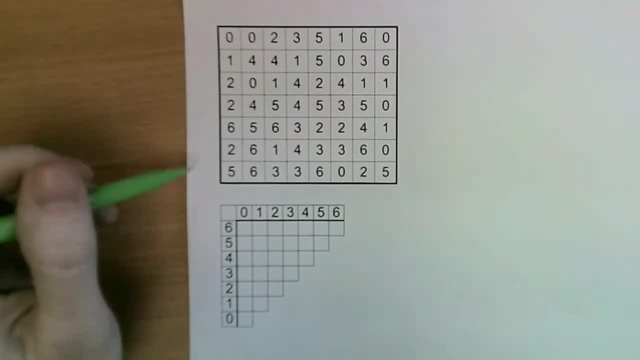 to mark off the dominoes so we can keep track of them as we place them. and we find the dominoes in this grid, and we'll simply put a bold line around each domino as we find it. Now. the typical way to solve these puzzles is to go through the dominoes in order, and 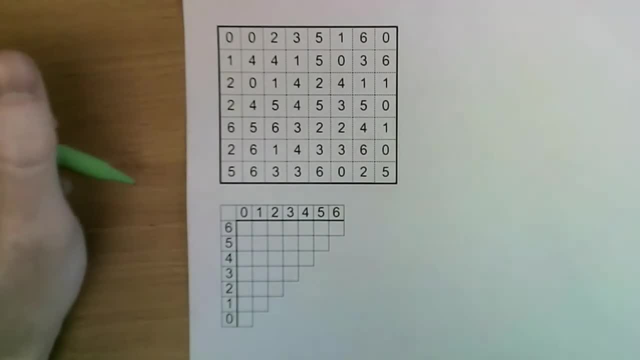 see if you can find a domino. that can only appear in one place in the grid, So let's start. So first of all, let's look for 0-0.. Okay, that's very handy. There's only one 0-0 in the grid, because these are the only. 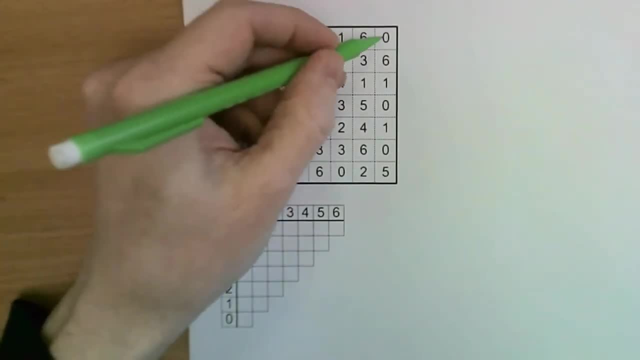 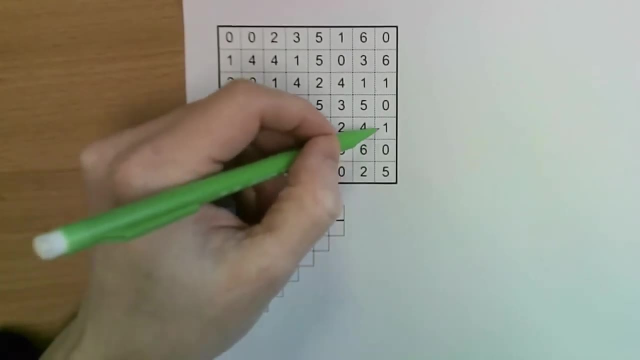 two 0s that neighbour each other. So that could be 0-6,, that could be 0-4,, that could be 0-1, that could be 0-5,, 0-2, 0-3, 0-6,, 0-6.. So anywhere the 0 neighbours another. 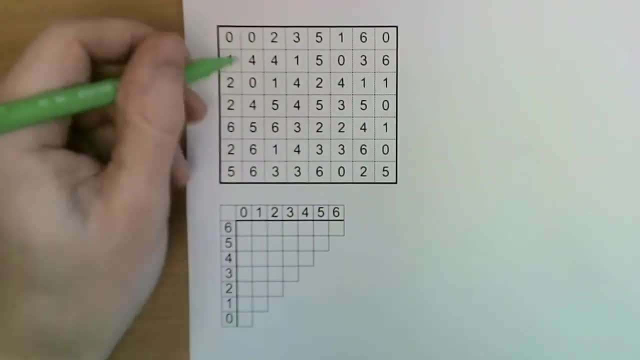 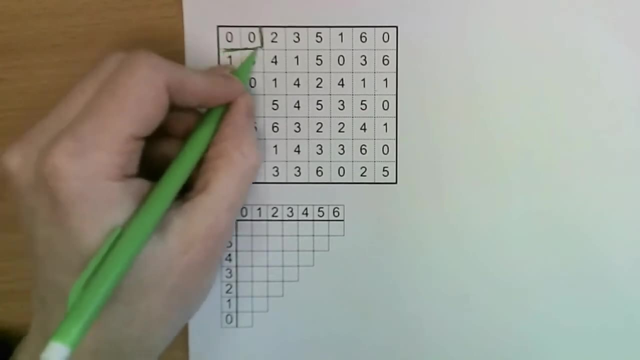 square horizontally or vertically is an option, but there's no other 0 that neighbours another 0. So that must be the 0-0.. So let's mark that in and let's pull across to show that we've placed that in the grid. Now I will continue doing that in a second, but just as I was. 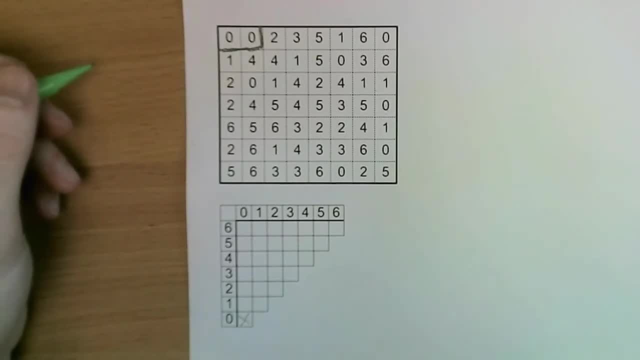 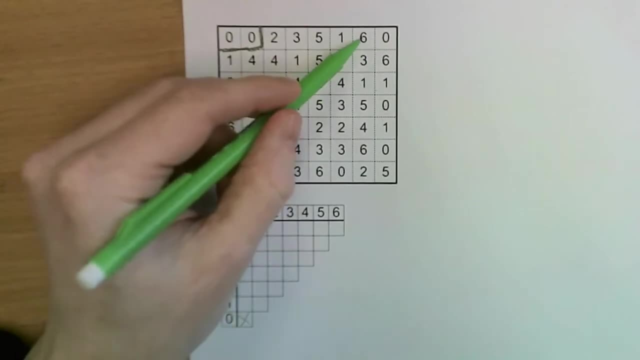 doing that, I saw another instance of a rule that can be used. So, if we look at this 0 in the corner, it has to pair to a 6.. So, whilst we don't know whether it goes to the left or whether it goes down, its only option is a 6.. 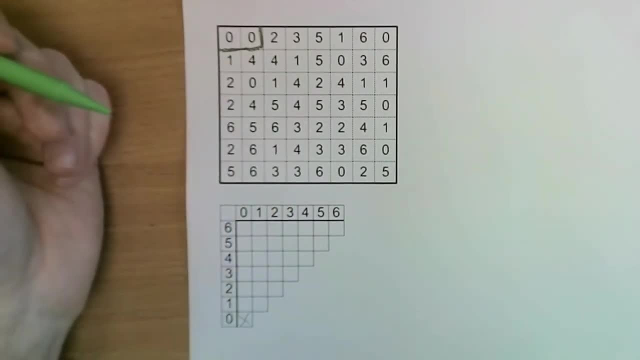 Therefore, you know, one of these two must be 0-6.. And so we can know that anywhere else in the grid that has 0-6 as an option cannot actually be that domino. So here we have 0 and 6 next. 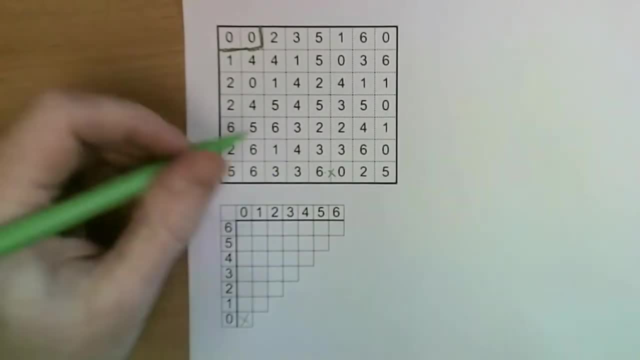 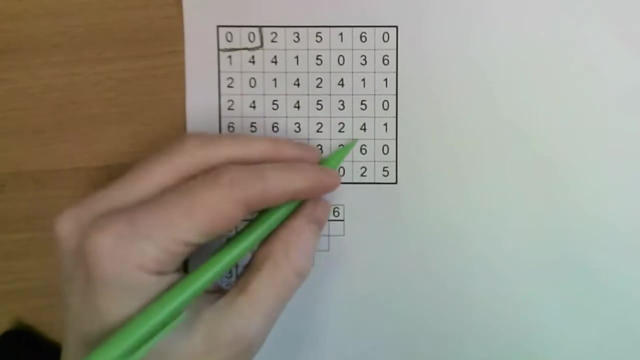 to each other. So we can put a little cross there to remind ourselves that it cannot be 0-6.. It has to be 0-3 or 0-2, because this has to be the 0-6 in some order. Likewise, 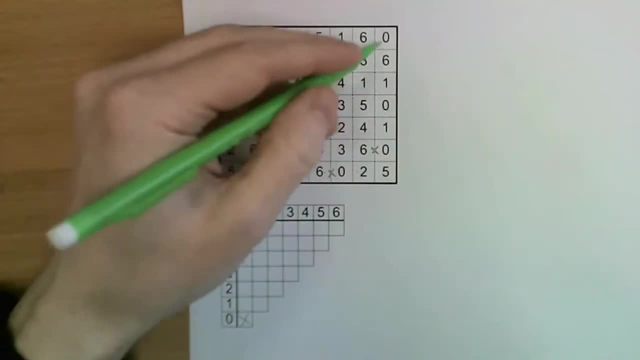 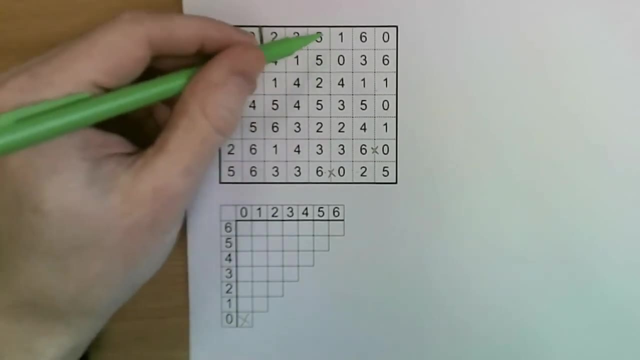 here. that cannot be the 0-6.. The 0-6, because it has to be at the top, Okay, so now I'm going to look for 0-1.. It can go there. It can go there, Okay, And as. 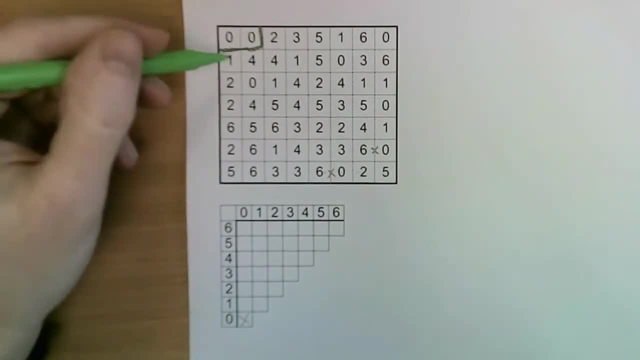 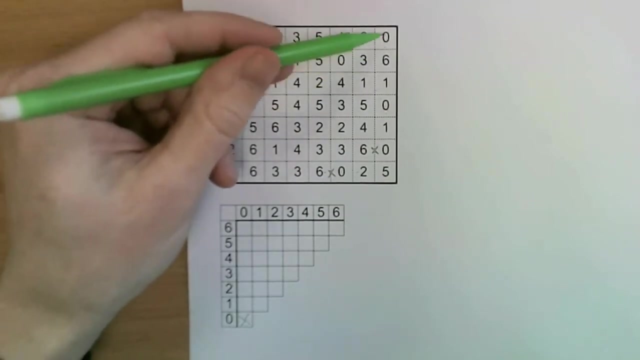 soon as you find two options, then you'd normally stop: 0-2,, 0-2,, 0-3,, 0-3,, 0-4,, 0-4,, 0-5,, 0-5.. And we know the 6-0 has to go up the top here. 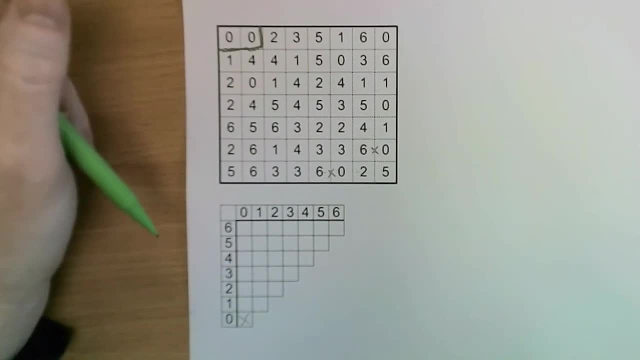 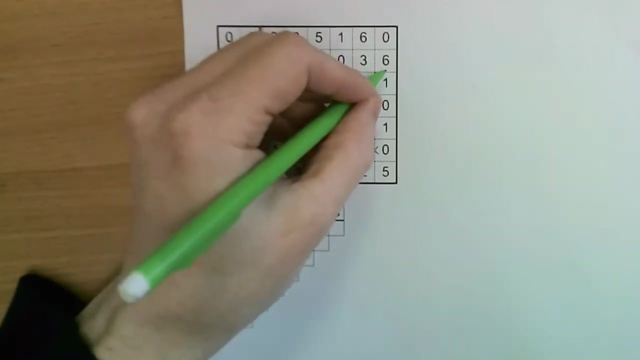 Okay, So let's move on to 1-0,, 1-0, 1-0.. Let's move to 1-1.. Okay, So it looks like here is the only possible instance of 1-1.. So let's mark that in. 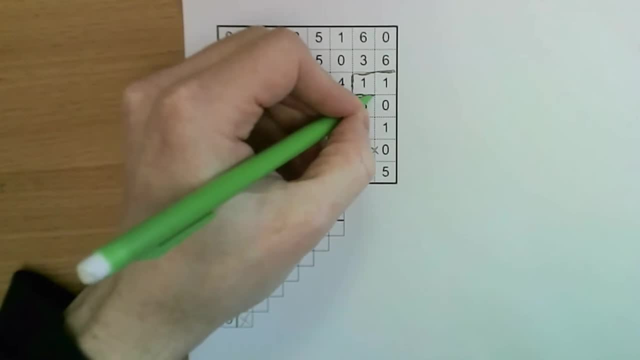 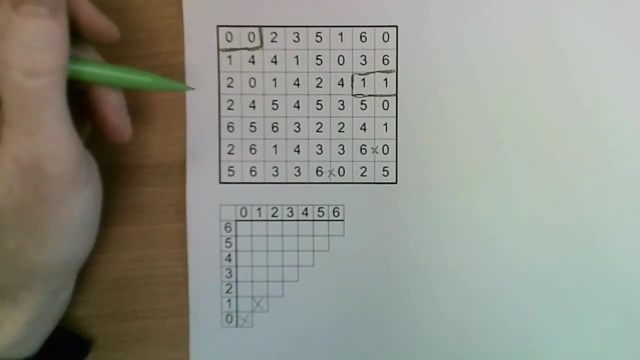 Now, as you start to place dominoes, you'll begin to restrict the possibilities for a lot of other placements, which hasn't happened yet, but that will hopefully happen fairly soon. So next let's look for 1-2.. So 1-2 here. That looks like the only option for the 1-2. 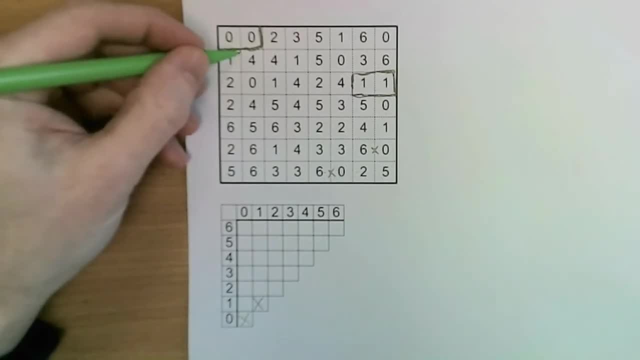 domino. Okay, great, So let's place that. Okay, I'll stick borders, just so it can be seen on the camera. 1-2.. Okay, Again, doesn't seem to immediately give us anything else. Let's keep going So. 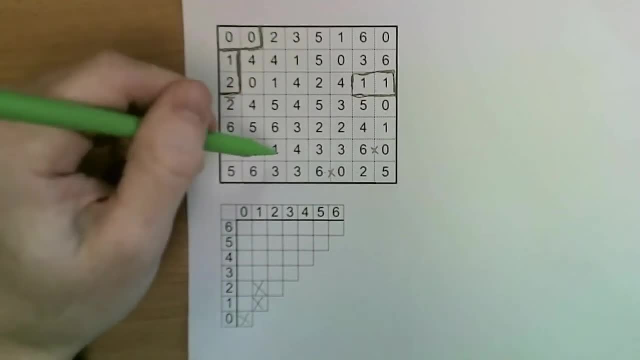 that was 1-2.. Let's try 1-3.. Go here there: 1-4,, 1-4,, 1-5,, 1-5,, 1-6,, 1-6.. Okay, So let's move on to 2-0 now. 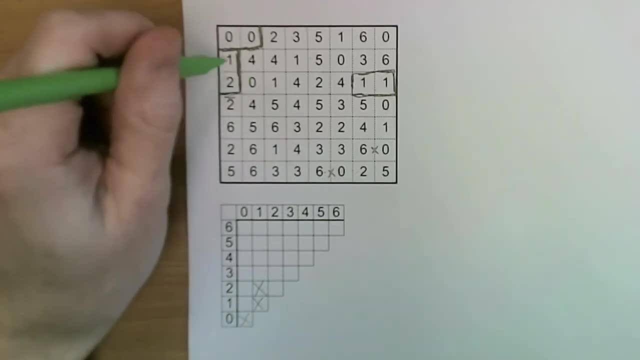 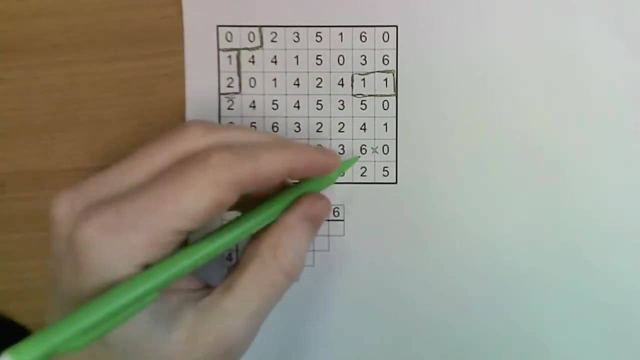 So originally this could have been 2-0, but now it can't be because we know the 2 is in this domino 2-0. Okay, So this must be the 2-0. So this 1-2 was actually useful because it ruled out. 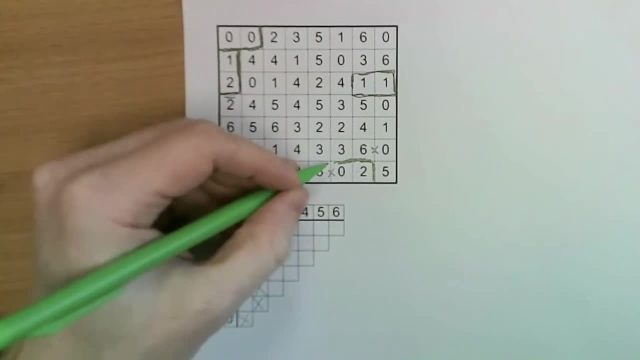 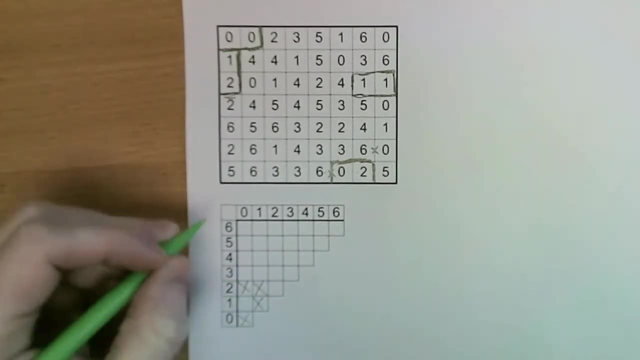 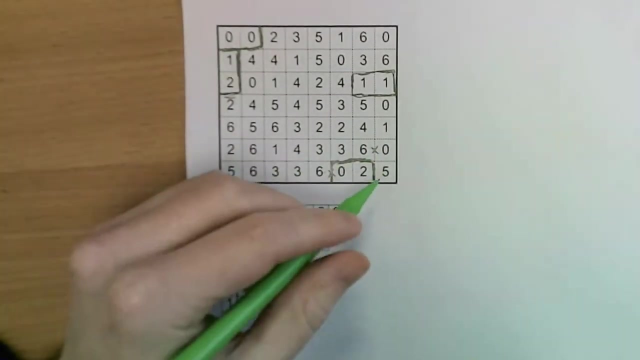 the 2-0 there. So that's going to be our 2-0, our 2-0.. Okay, So now we have our first instance where we can, We can mark something else straight away now. So this 5. now the corner squares were very. 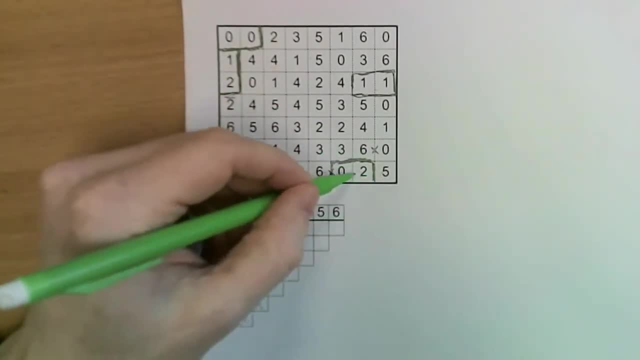 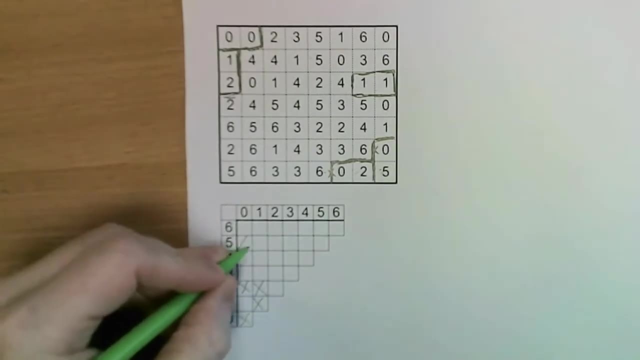 restricted of course. They only have two possible squares they can connect to. And now it can't go here, It must come out here. So this is our 5-0.. So that's 5-0.. So let's keep going from 2-2.. Let's look for 2-3.. 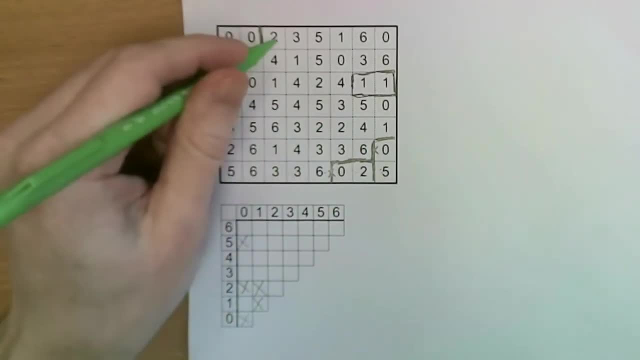 Okay, So that could be 2-3, 2-3,, 2-3,, 2-4,, 2-4.. 2-5,, 2-5,, 2-6.. Okay, So not there or there. Here could be 2-6.. That could be 2-6.. Okay, fine. 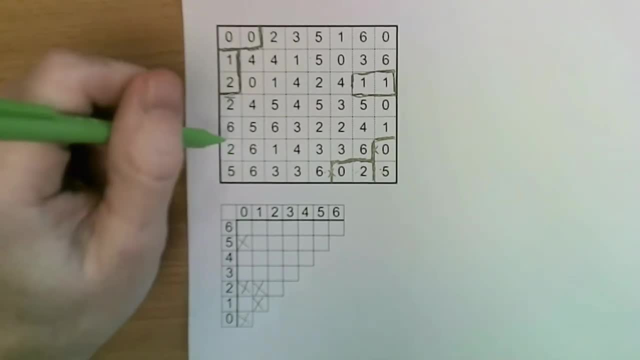 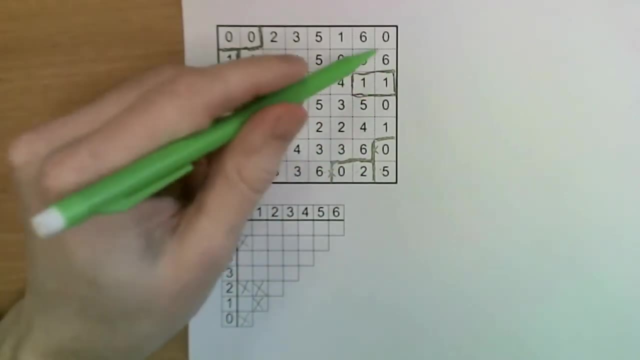 So nothing doing there. Let's move on to the 3.. So let's look at 3-0.. Okay, So can't go there. Looks like it's here 3-0.. So let's mark that in. 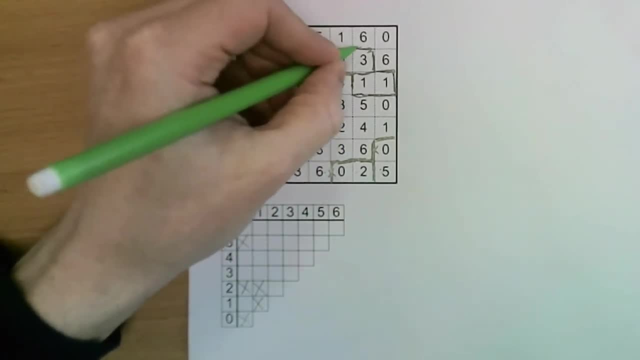 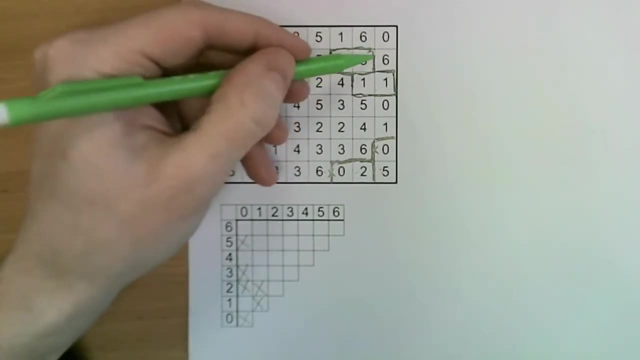 Okay, That's going to give us more information as well, which is great. So that's the 3-0 or 0-3.. So now you can see that we can resolve our 6-0, because this 6 can no longer neighbour. 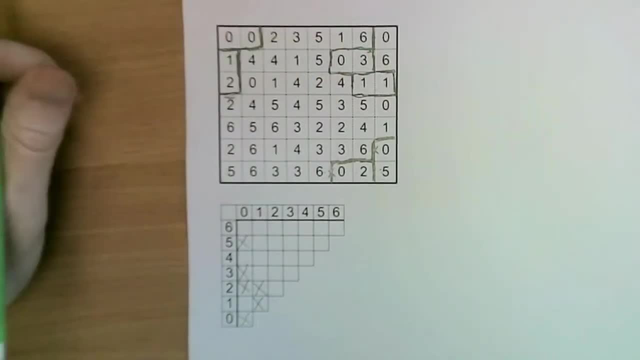 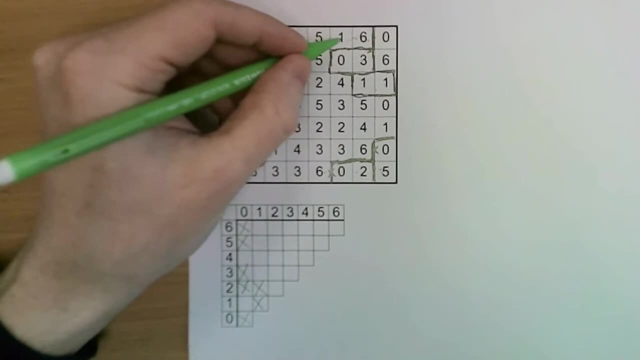 the 3 or the 1.. So it must neighbour the 0 there. So that's the 6-0 marked in. Let's check that. And that also gives us the 6-1.. Okay, Because now this 6 has to connect to this 1.. So that's the 6-1.. 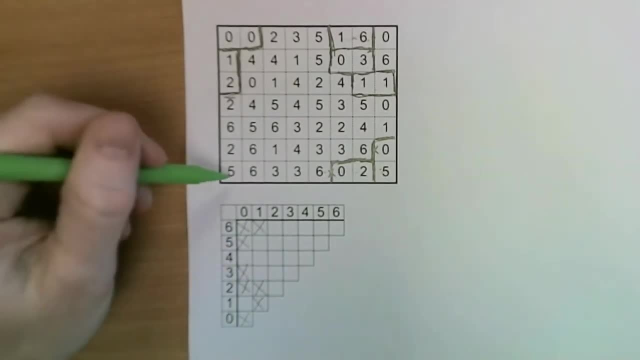 Okay, So let's continue. Let's look at 3-1.. 3-1,, 3-1,, 3-2, there, there, 3-3, here or here. 3-4, there or there, 3-5, there or there, 3-6, there or there. Okay, all there, Let's look. 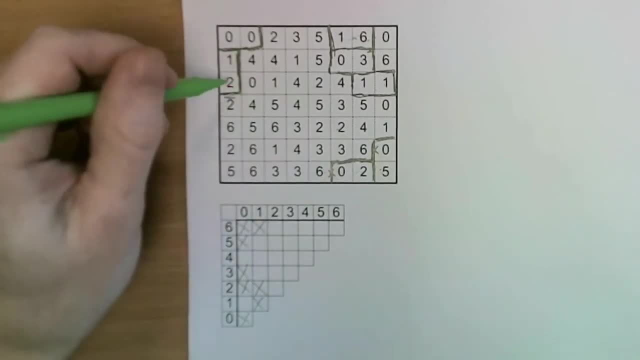 at 4-0.. So 4-0. Okay, So it's either this 4 or this 4 connected to the 0. But we don't know which. 1 yet 4-1, lots of options. 4-2, there there, 4-3, there there, 4-4, looks like. 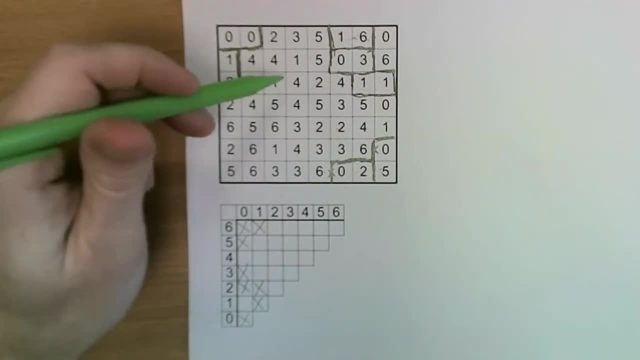 it's only here in the middle of the grid. Let's just check that. Hold on 4,. no, could be there. Okay, Almost moved too quickly there. 4-5.. 4-5,, 4-5, lots of options for. 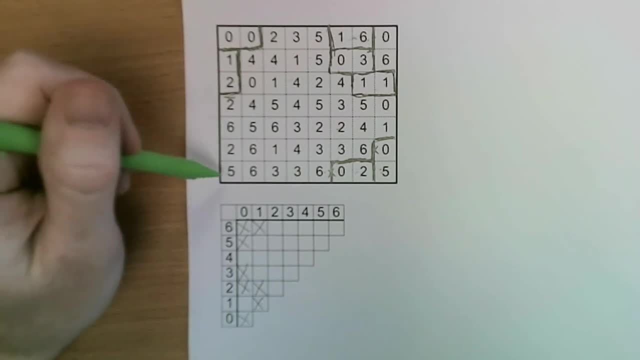 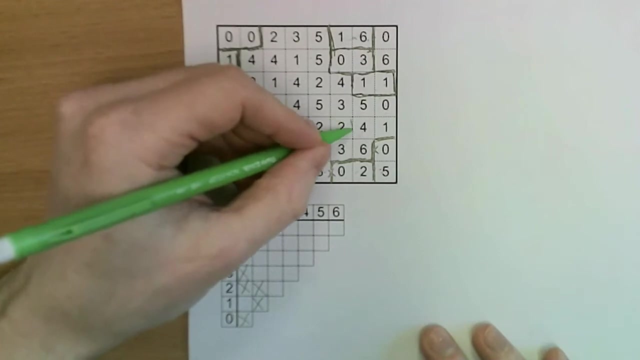 4-5.. Let's move on to 4-6.. So we have an option here: 4-6.. Do we have any others? Let's just check. No, no, no, no, no. Okay, So this is 4-6.. 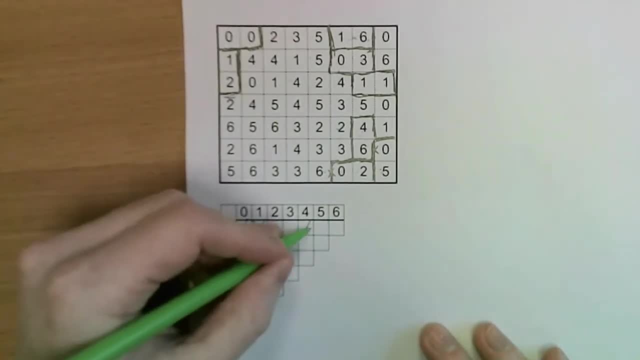 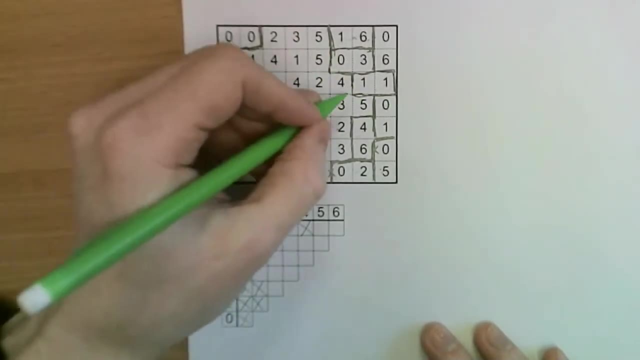 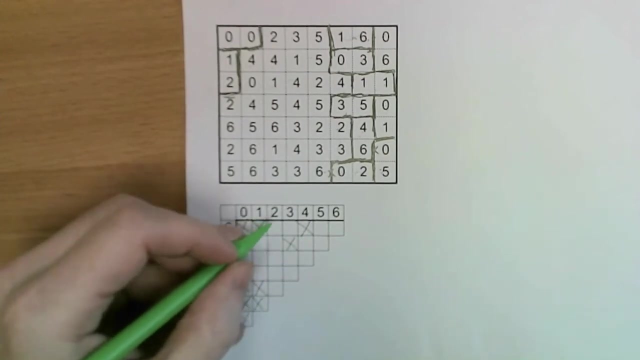 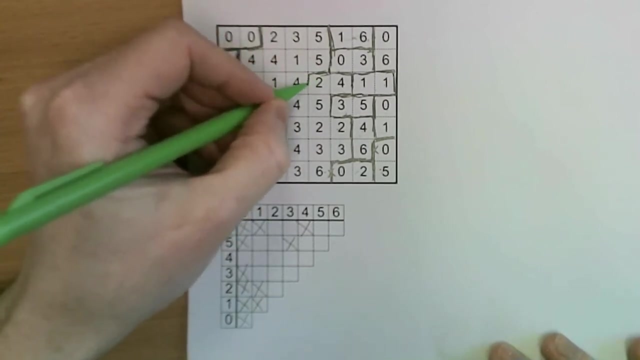 4-6,, 6-4.. Okay, This also gives us another couple of freebies. So here's our 0-1.. And here's our 5-3.. 5-3.. Now, that actually also gives us this 4-2.. So that's 4-2.. 4-3,, 4-2,. 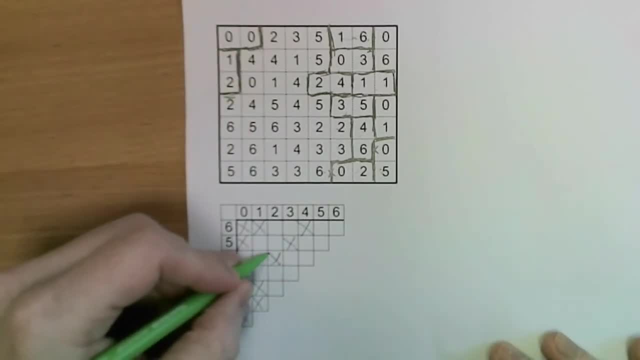 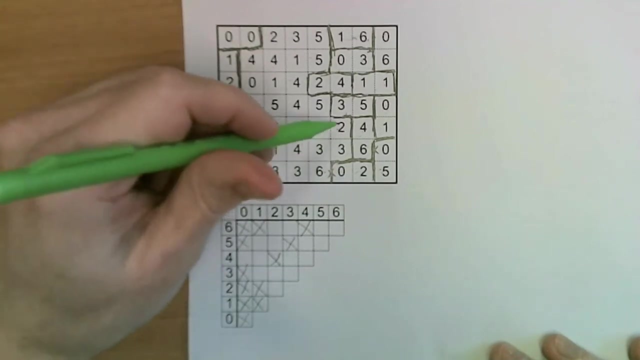 4-2.. 4-2.. 4-2.. 4-2.. So let's move on to looking at the 5s now. So 5-0, we already have placed. So let's look at 5-1.. So 5-1.. Could be here, could be here 5-2, here, here, 5-3. we've already. 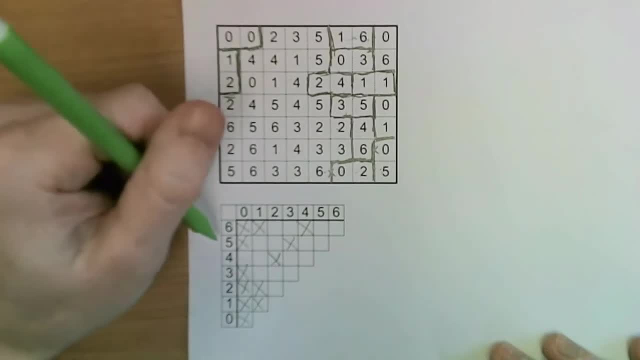 placed 5-4,, there, there, 5-5,. let's have a look at 5-5.. 5-5 can only be placed here, only go here. so that's the five, five, five, five. and now let's move on to the sixes. so six, zero and six, one already placed. this is where 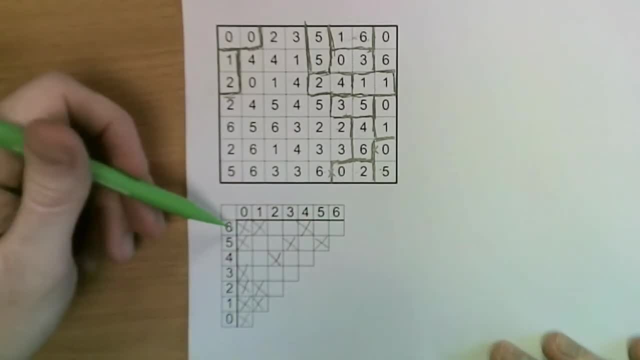 this. this grid gets um gets useful for checking what we've already placed um six two. so six, six two. six three, six five. so this must be the six two um, that's the only option for it. um, no, again too quick. six two, six two or six two, so um always worth double checking. six three. 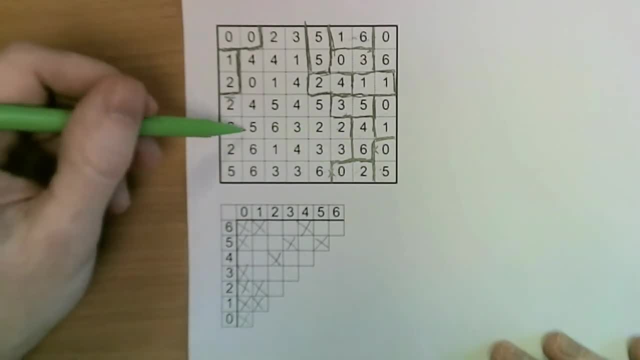 six, four. we've already placed that, i believe. yes, six, five, here we're here. how about the double six? not there, not there, not there. okay, that must be down here. just double check in again. um, yep, okay, fine, six, six, the easiest way to go wrong. um, in solving dominoes, as i've almost shown a couple of times, 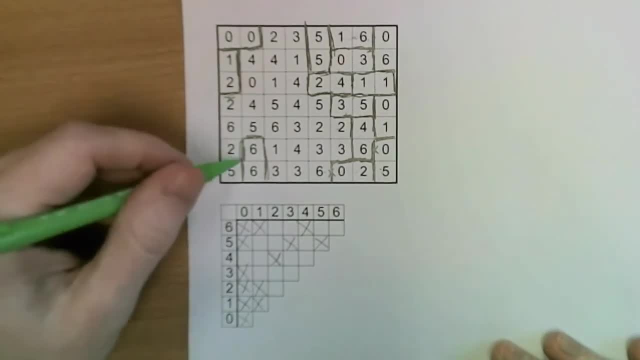 is to skip over a potential placement and therefore marking the one one. so that's six, six. that gives us the two, five or the five. two, um, okay, now we'll just go round again and start looking at the dominoes that we haven't placed yet. um, and hopefully some of these. 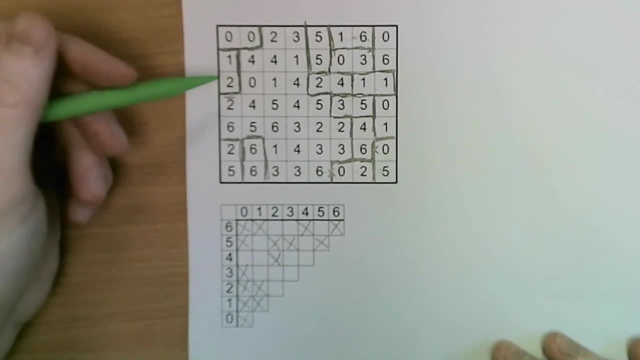 place dominoes will have now resolved some that we couldn't place before. so let's come back around to the lowest one, which is two, two. so where can that go? so two, three is two. sixty four. so two, two. okay, so that must now be over here. so that's the two, two. 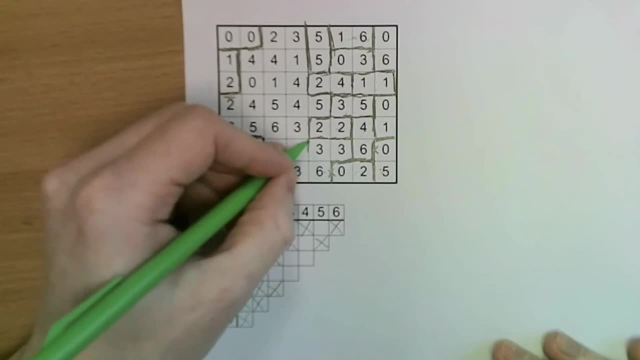 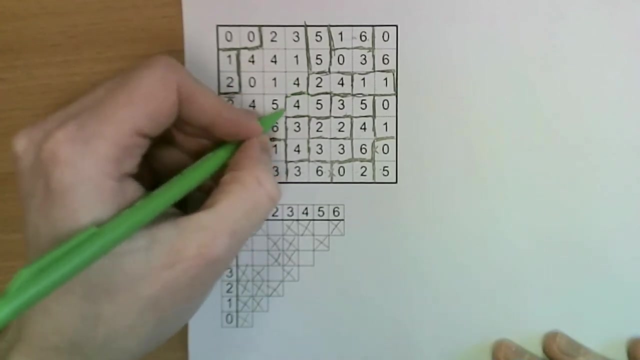 two, two. that gives us a three, three, three, three. that in turn gives us the six, three. and you can see that as you replace more and more um, the grid just starts to resolve itself. that gives us this three, one that gives us the four, three, four, three. that gives us the five, four, and, like a lot of puzzles, it builds momentum, um, like this: